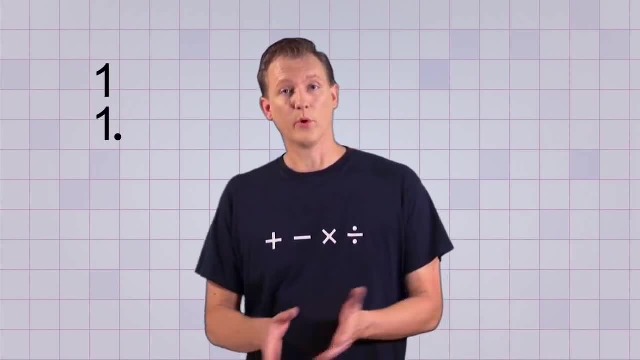 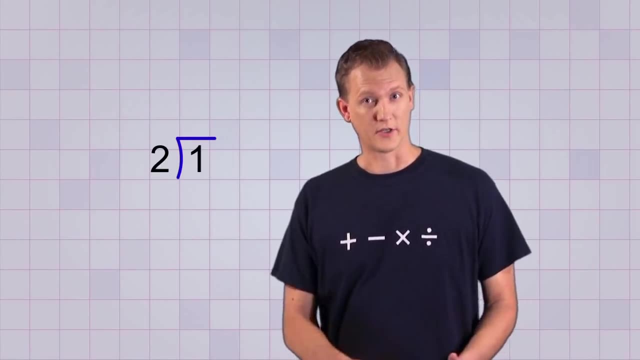 Now you remember that in the last section we learned that 1 could be written as 1.0, or 1.00, or 1.000, and its value is still 1.. Let's try doing that here and see what happens. 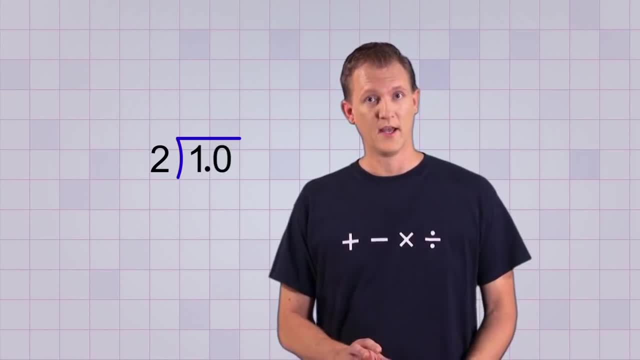 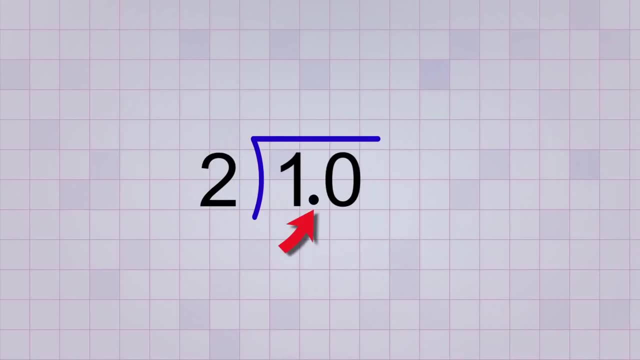 After the 1, put a decimal point and then a 0 in the tenths place. Now our division problem looks like 10 divided by 2. And that's easy to do. The only difference is we have a decimal point. Let's ignore the decimal point for a minute. 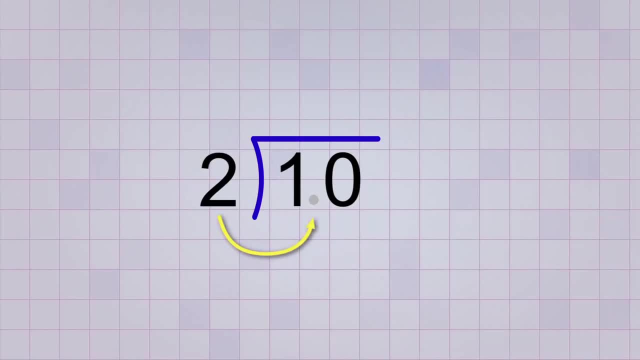 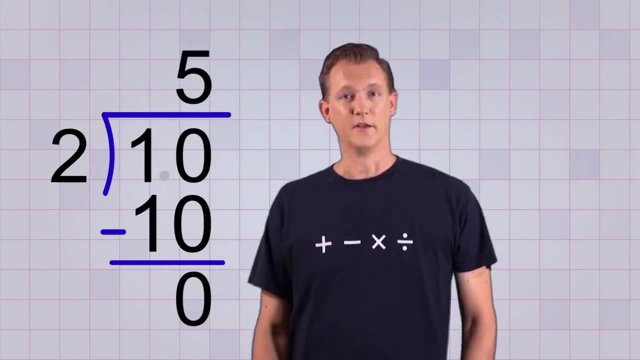 knowing that our problem really is 10 divided by 2. So 2 will go into 10 five times, because 5 times 2 equals 10. And that leaves no remainder. So we're done right, Not so fast. We've got that decimal point to deal with. 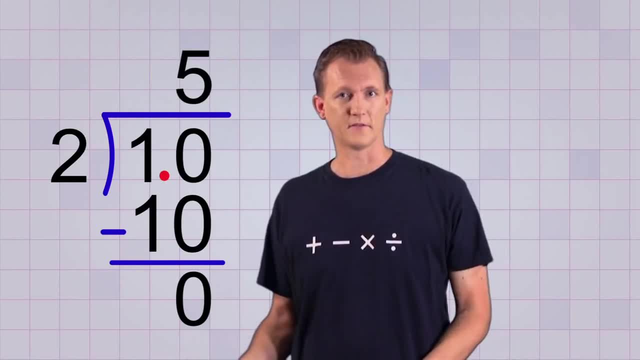 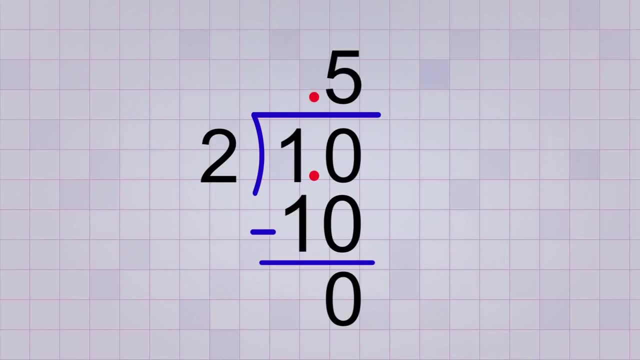 And we know that 5 can't be the answer because 5 is bigger than 1 half. We just need to include the decimal point in our answer for it to be correct. We put it directly above the decimal point in our problem. 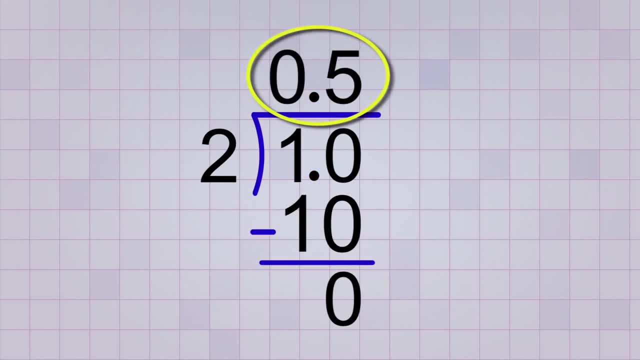 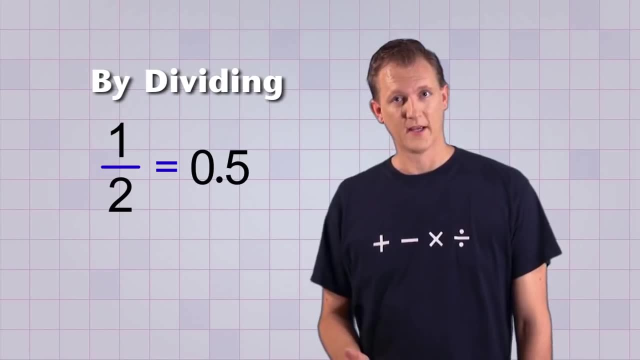 There. Now. our answer is .5, or 0.5, which is the more proper way to write it. So by dividing we figured out that the decimal value of 1 half is 0.5.. Now let's try converting the fraction 3 fourths by dividing. 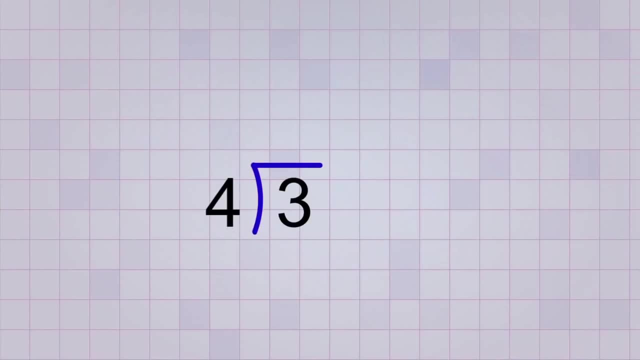 Of course, we start by rewriting our fraction like this: 3 divided by 4.. And again we run into the same problem: 4 is too big to go into 3.. So it looks like we're going to need a decimal point here too. 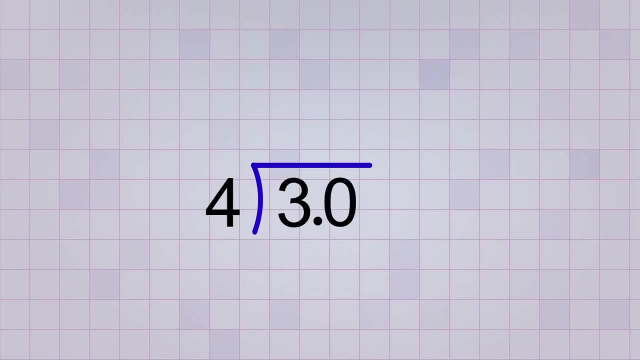 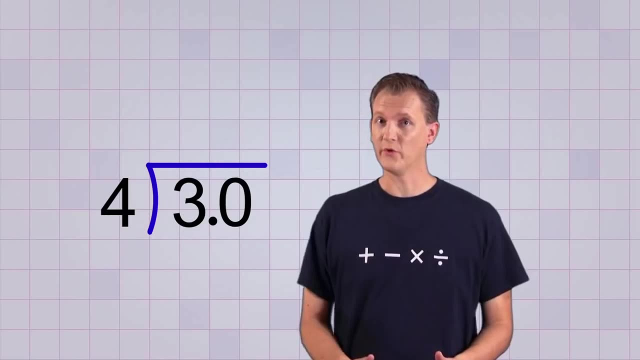 Let's put a decimal point after the 3 and a 0 in the tenths place to make 3.0.. Now our problem almost looks like 30 divided by 4.. Now if you remember your multiplication table, you'll know that 4 goes into 30 seven times. 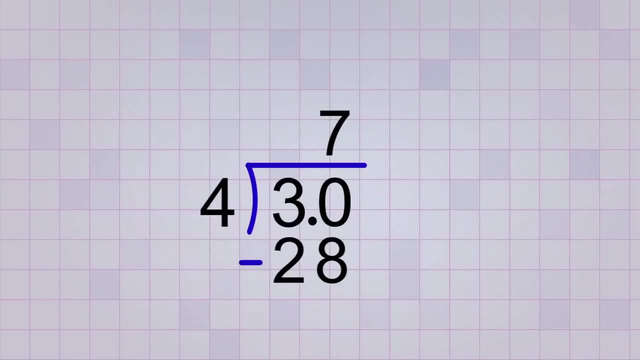 because 7 times 4 is 28.. 30 minus 28 leaves a remainder of 2, but we don't want a remainder, so let's keep going. 4 is too big to divide into 2, so the only way we can get rid of the remainder 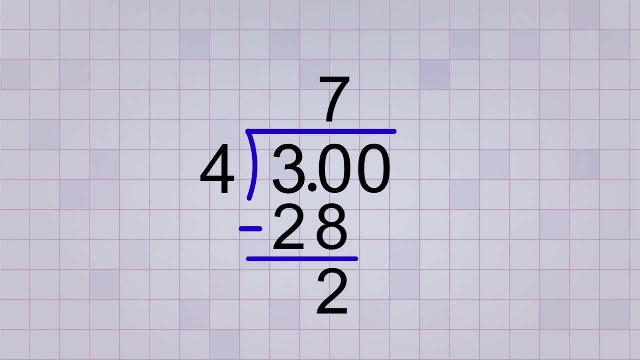 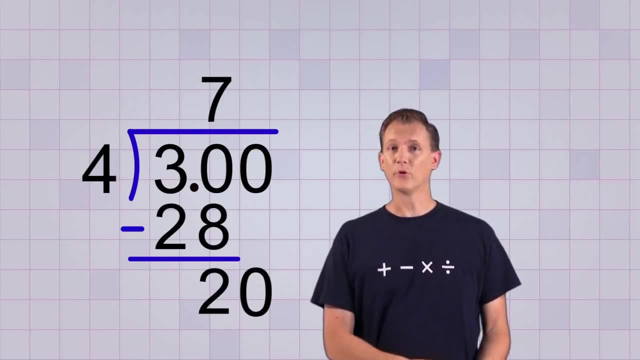 is to use another 0 in the hundredths place, which makes the number we're dividing up kind of look like 300.. Now we can bring down that extra 0 to make the remainder look like 20.. And 4 will go into 20 five times. 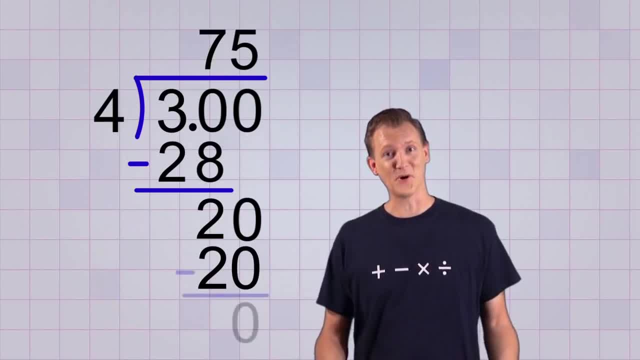 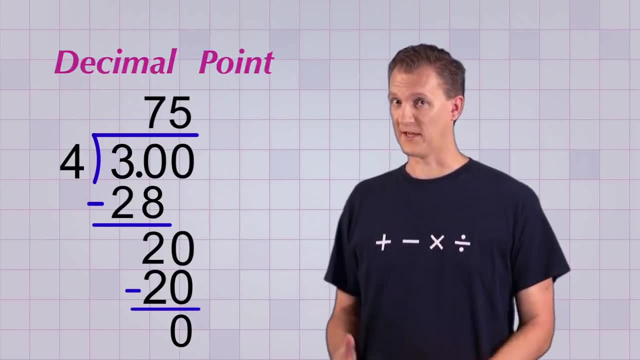 because 5 times 4 equals 20, and that leaves no remainder. Oh yeah, But don't forget, we need to include the decimal point in our answer. Now, if you've kept your columns lined up, like I have, you'll see that the decimal point goes right here. 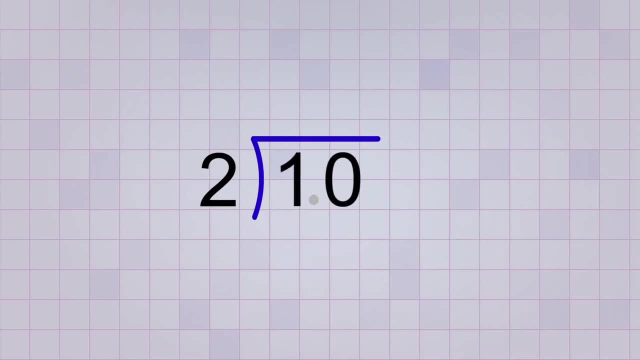 Let's ignore the decimal point for a minute, knowing that our problem really is 10 divided by 2.. So 2 will go into 10 five times, because 5 times 2 equals 10. And that leaves no remainder. So we're done, right. 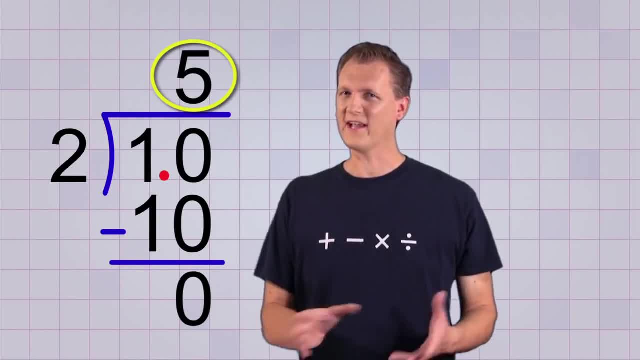 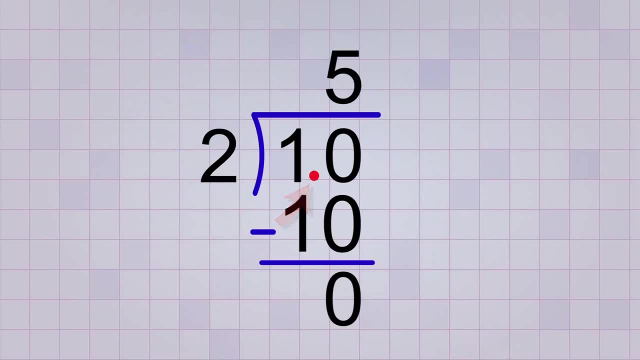 Not so fast. We've got that decimal point to deal with And we know that 5 can't be the answer because 5 is bigger than 1 half. We just need to include the decimal point in our answer for it to be correct. 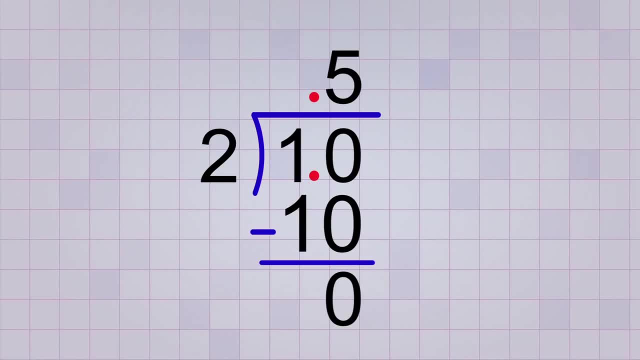 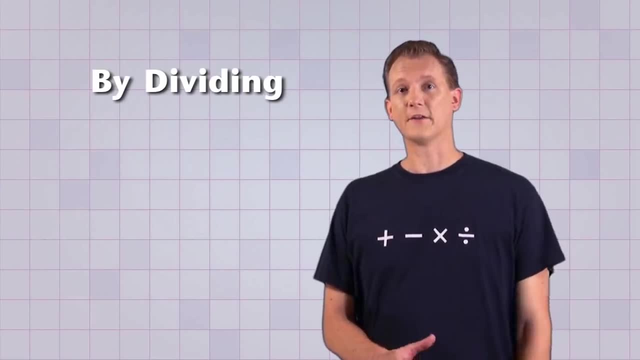 We put it directly above the decimal point in our problem. There Now, our answer is .5, or 0.5, which is the more proper way to write it. So by dividing we figured out that the decimal value of 1 half is 0.5.. 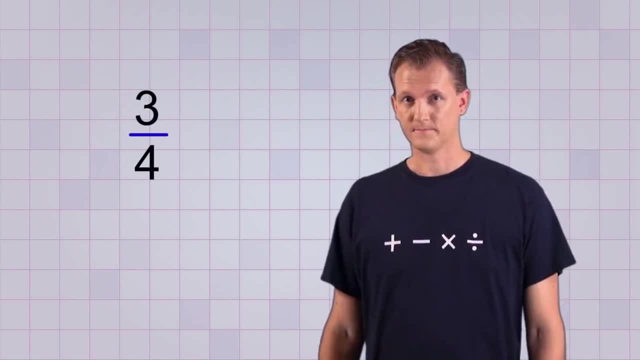 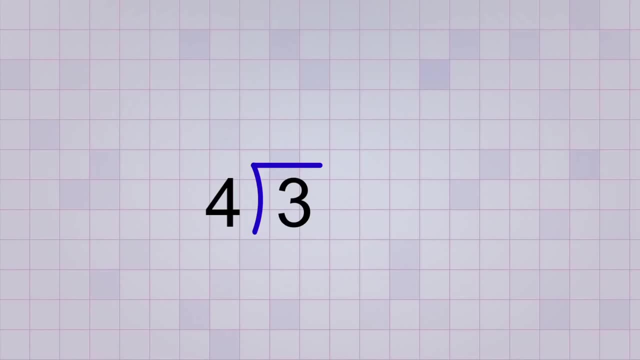 Now let's try converting the fraction 3- fourths by dividing. Of course we start by rewriting our fraction like this: 3 divided by 4.. And again we run into the same problem: 4 is too big to go into 3.. 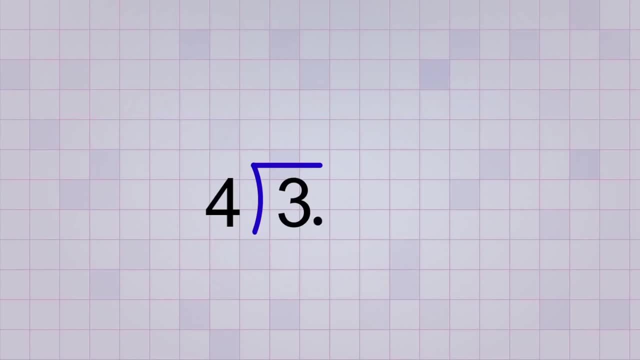 So it looks like we're going to need a decimal point here too. Let's put a decimal point after the 3 and a 0 in the tenths place to make 3.0.. Now our problem almost looks like 30 divided by 4.. 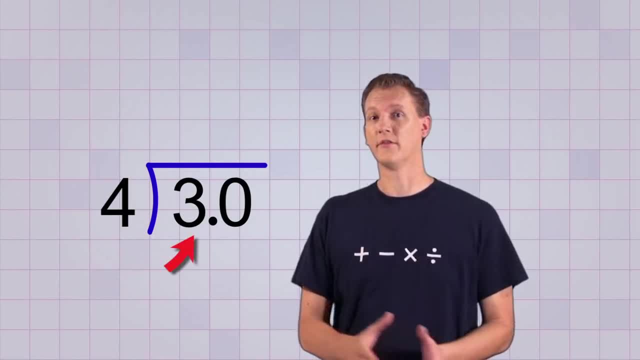 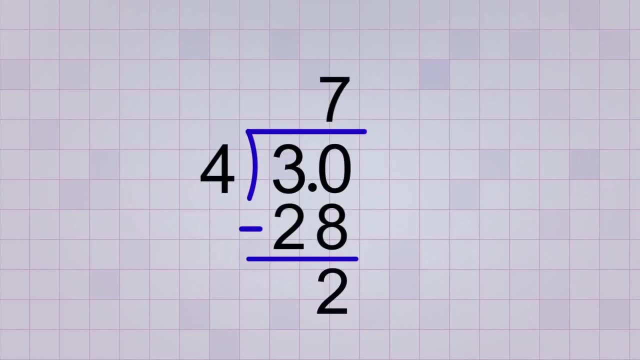 Now, if you remember your multiplication table, you'll know that 4 goes into 30 seven times, because 7 times 4 is 28.. 30 minus 28 leaves a remainder of 2, but we don't want a remainder, so let's keep going. 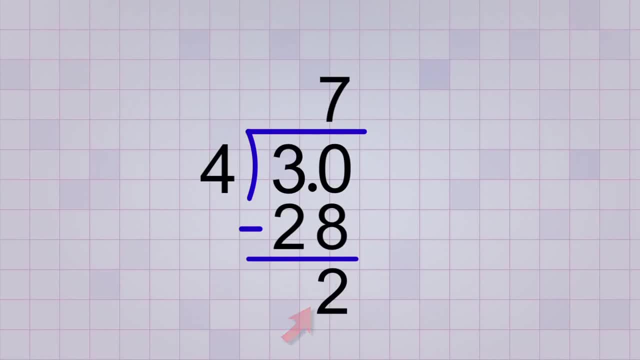 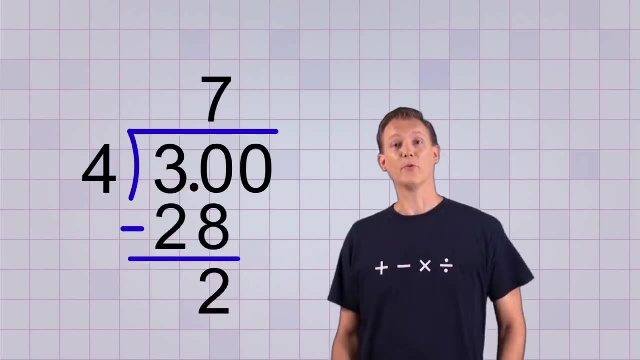 4 is too big to divide into 2, so the only way we can get rid of the remainder is to use another 0 in the hundredths place, which makes the number we're dividing up kind of look like 300.. Now we can bring down that extra 0 to make the remainder look like 20.. 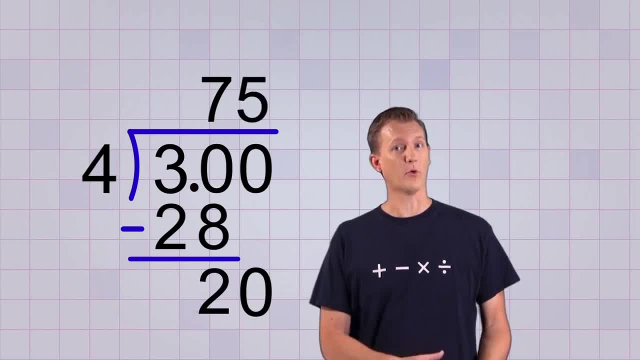 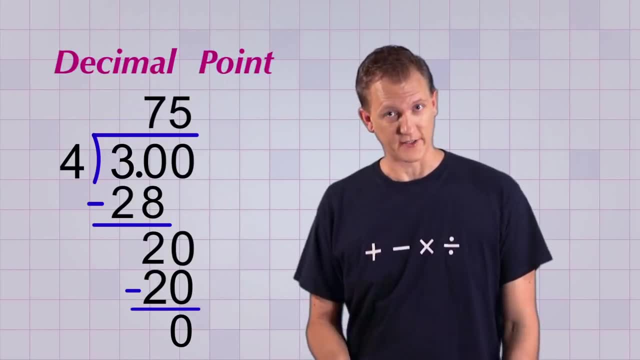 And 4 will go into 20 five times, because 5 times 4 equals 20, and that leaves no remainder. Oh yeah, But don't forget, we need to include the decimal point in our answer. Now, if you've kept your columns lined up like I have, you'll see that the decimal point goes right here. 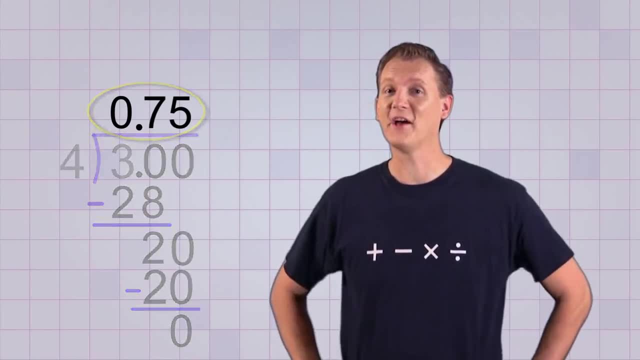 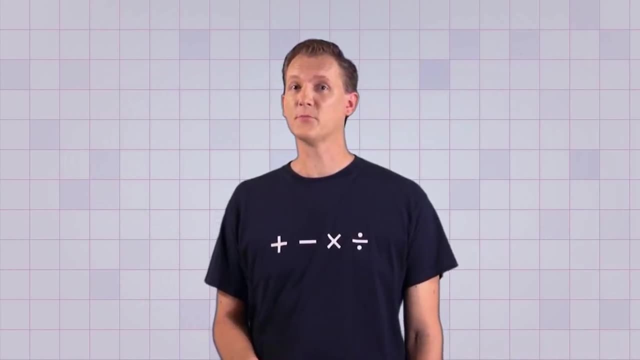 and that makes our answer 0.75.. So the decimal value of 3 fourths is 0.75.. Alright, let's convert one more the hard way. Let's find the decimal value of 1 third by dividing 1 by 3.. 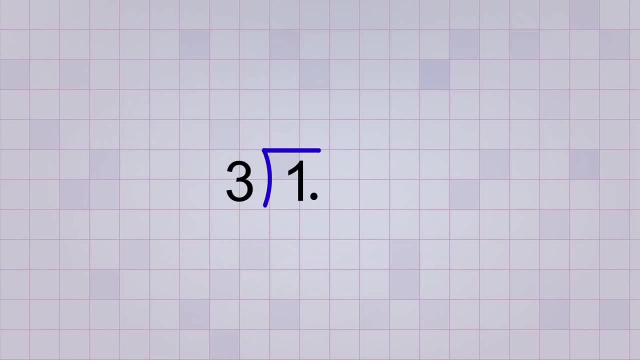 Again, 3 is too big to divide into 1, so we'll need to use a decimal point and another 0, which makes our problem look like 10 divided by 3.. That's easy: 3 goes into 10 three times. 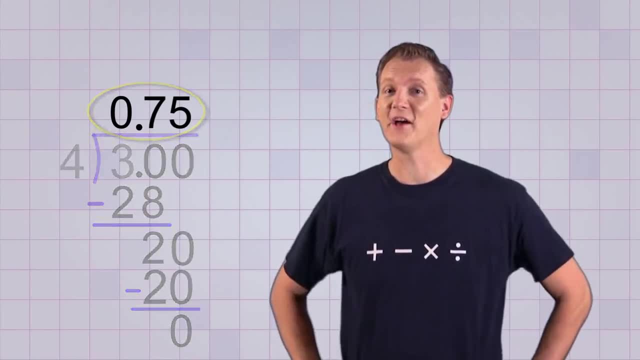 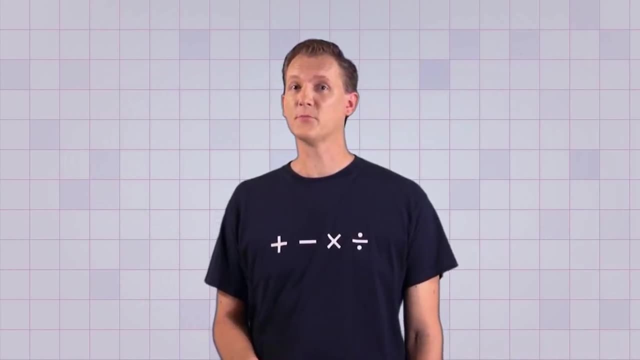 and that makes our answer 0.75.. So the decimal value of 3 fourths is 0.75.. Alright, let's convert one more the hard way. Let's find the decimal value of 1 third by dividing 1 by 3.. 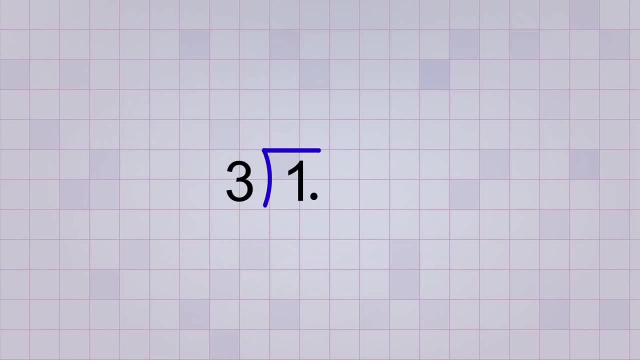 Again, 3 is too big to divide into 1, so we'll need to use a decimal point and another 0, which makes our problem look like 10 divided by 3.. That's easy: 3 goes into 10 three times. 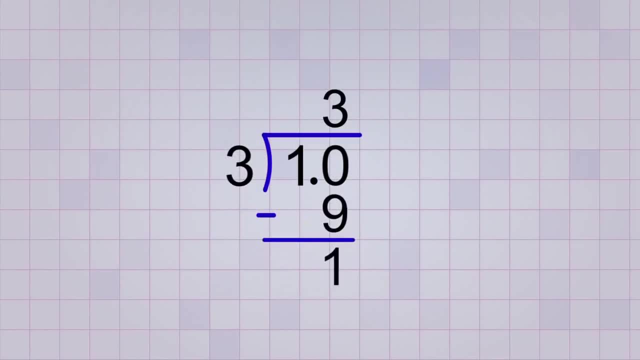 because 3 times 3 equals 9, and that leaves a remainder of 1.. Just like before, we don't want a remainder, so let's use another 0, so we can keep on dividing, And that gives us 10 divided by 3 again. 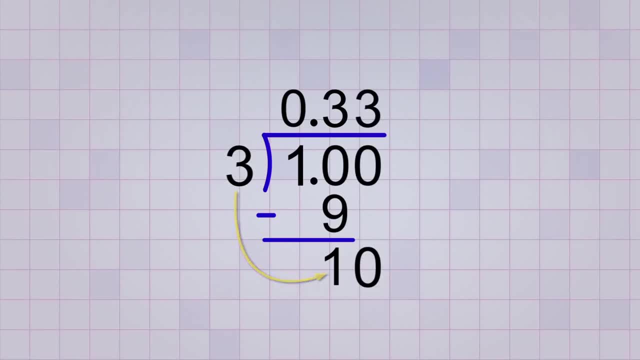 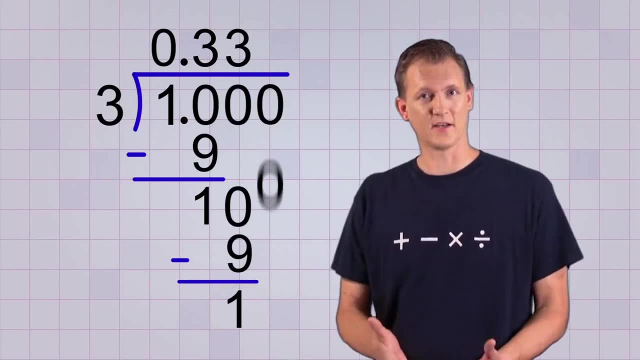 Well, we know that 3 goes into 10 three times and leaves a remainder of 1.. Huh, Still a remainder of 1.. Well, it looks like we're going to need another 0, but that's just going to give us 10 divided by 3 again. 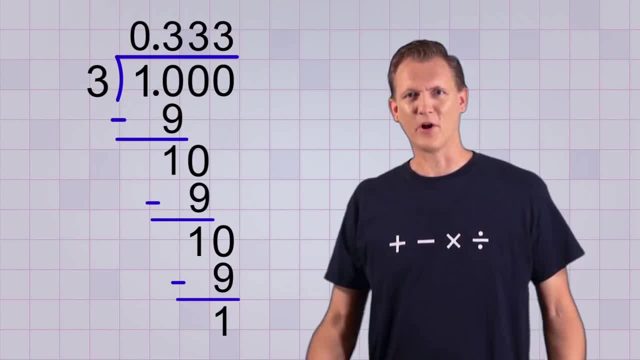 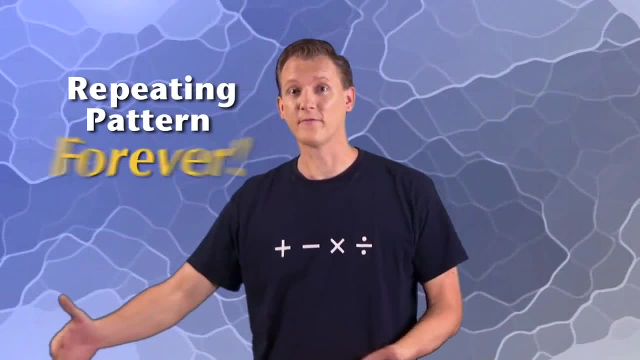 which is going to give us another remainder of 1.. This looks like it might keep on going forever. Some fractions are like that: If you divide them, you'll see a repeating pattern of numbers that continues on forever. So the decimal value of 1 third is 0.333333333,. 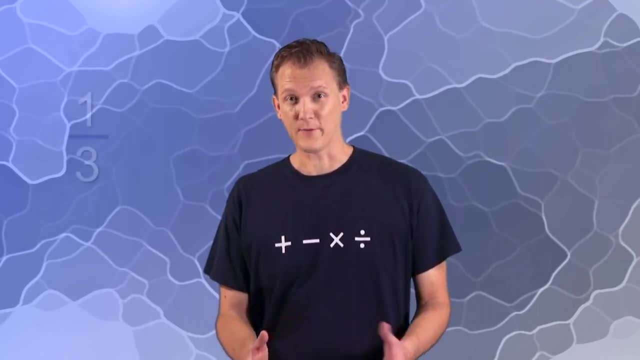 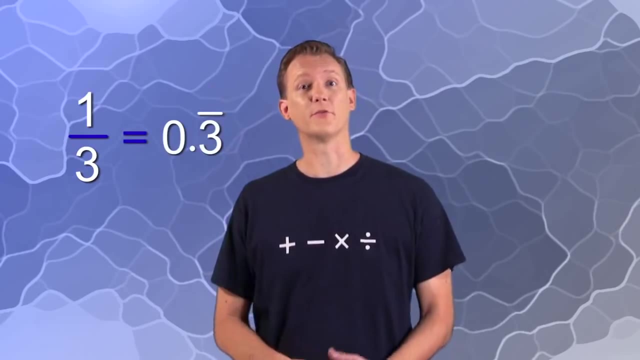 and 3's that keep on going forever. But since we can't keep writing 3's forever, we can just stop and round the number off, Or we can use this special symbol that means this number repeats forever. Alright, so all we have to do to convert a fraction. 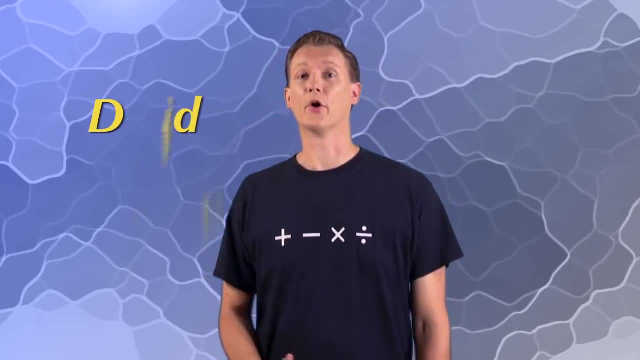 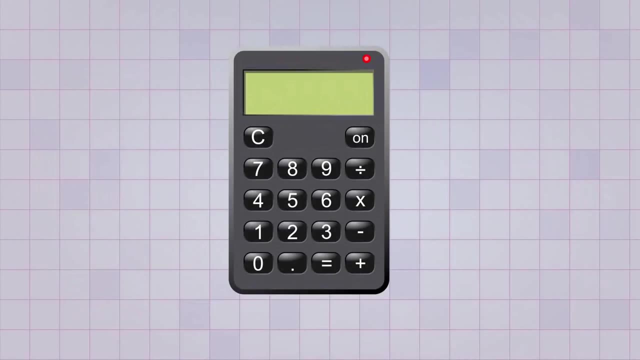 into a decimal is divide, And so far we've been doing that the hard way. But now we're going to do it the easy way. We're going to use a calculator. Let's try a couple with a calculator and see what we get. 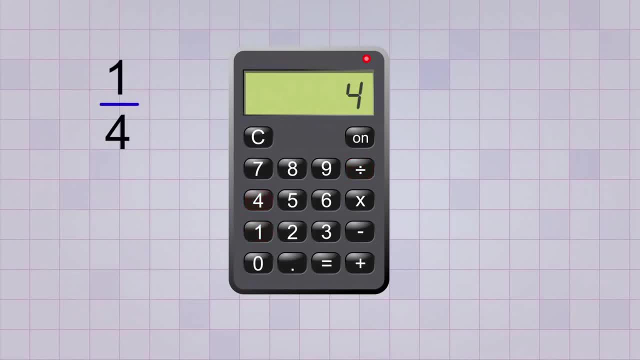 To convert 1 fourth, we just punch in 1 divided by 4, and we get 0.25.. To convert 2 thirds, we just punch in 2 divided by 3, and we get 0 point: a whole lot of 6's. 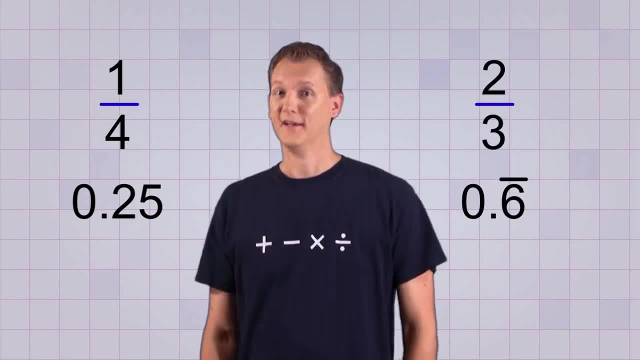 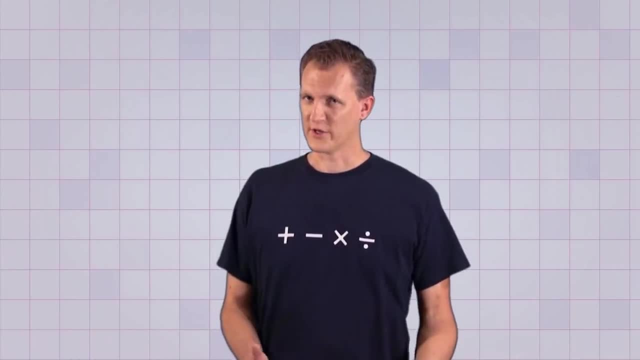 Looks like we have another one of those repeating decimals. Yep, this way's certainly easier and quicker too, But it's important to know how to do it both ways. The 5 fractions that we've just converted are so common that it's a good idea to memorize their decimal values. 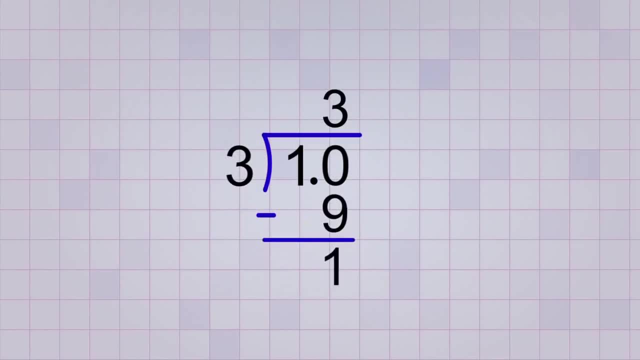 because 3 times 3 equals 9, and that leaves a remainder of 1.. Just like before, we don't want a remainder, so let's use another 0, so we can keep on dividing, And that gives us 10 divided by 3 again. 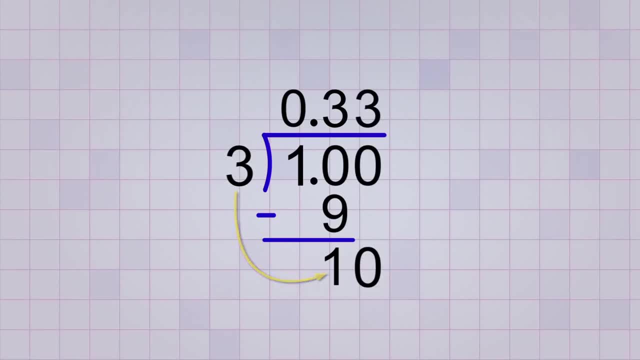 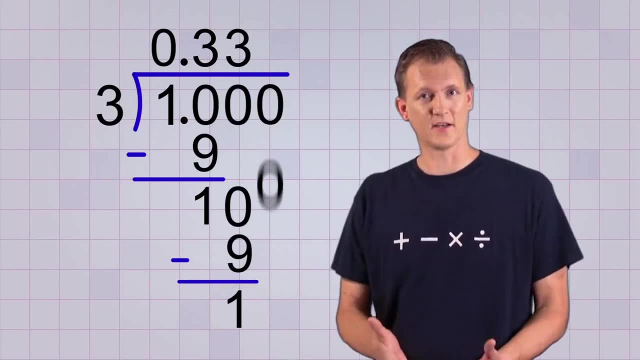 Well, we know that 3 goes into 10 three times and leaves a remainder of 1.. Huh, Still a remainder of 1.. Well, it looks like we're going to need another 0, but that's just going to give us 10 divided by 3 again. 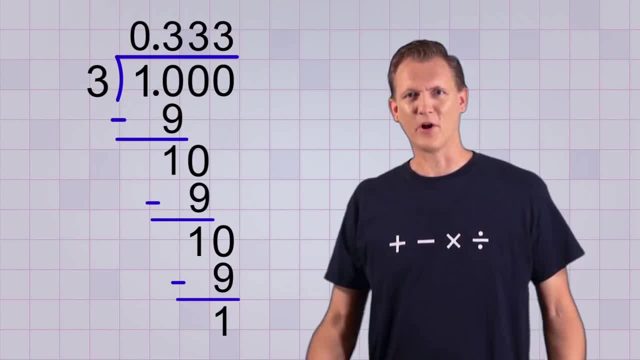 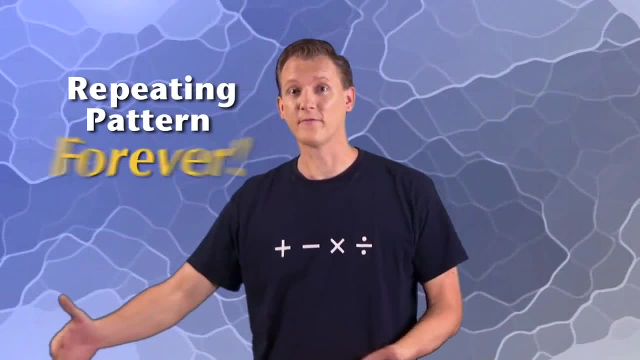 which is going to give us another remainder of 1.. This looks like it might keep on going forever. Some fractions are like that: If you divide them, you'll see a repeating pattern of numbers that continues on forever. So the decimal value of 1 third is 0.333333333,. 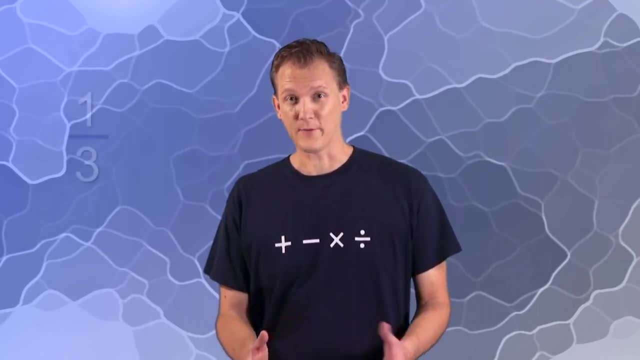 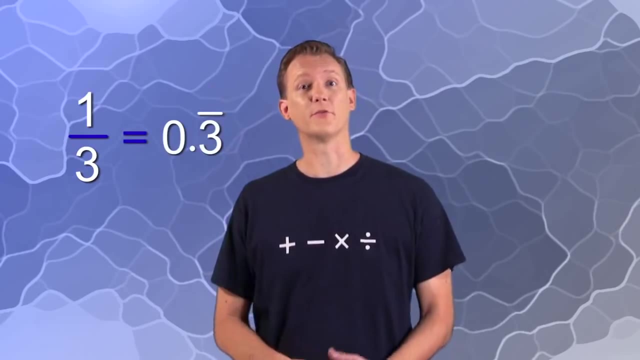 and 3's that keep on going forever. But since we can't keep writing 3's forever, we can just stop and round the number off, Or we can use this special symbol that means this number repeats forever. Alright, so all we have to do to convert a fraction. 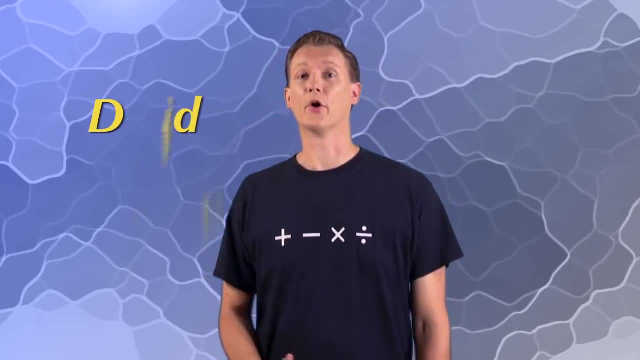 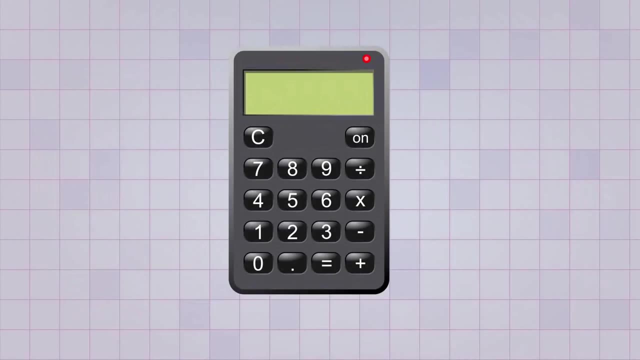 into a decimal is divide, And so far we've been doing that the hard way. But now we're going to do it the easy way. We're going to use a calculator. Let's try a couple with a calculator and see what we get. 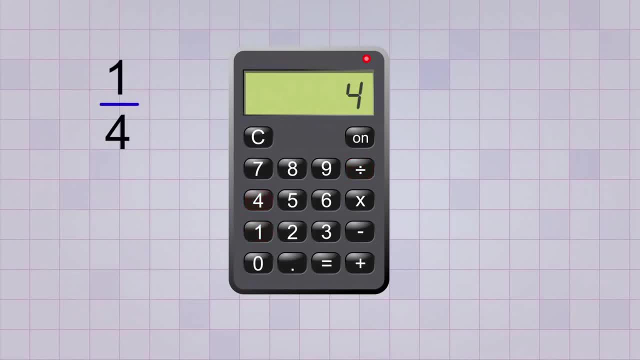 To convert 1 fourth, we just punch in 1 divided by 4, and we get 0.25.. To convert 2 thirds, we just punch in 2 divided by 3, and we get 0 point: a whole lot of 6's. 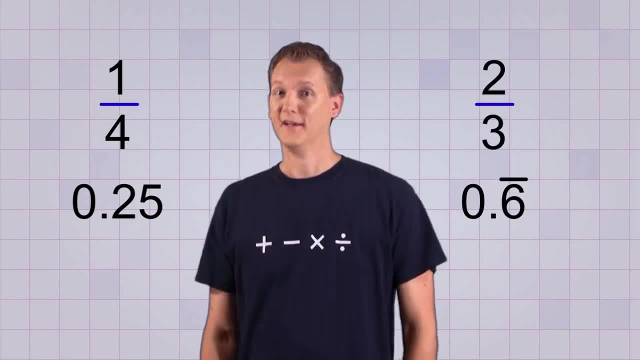 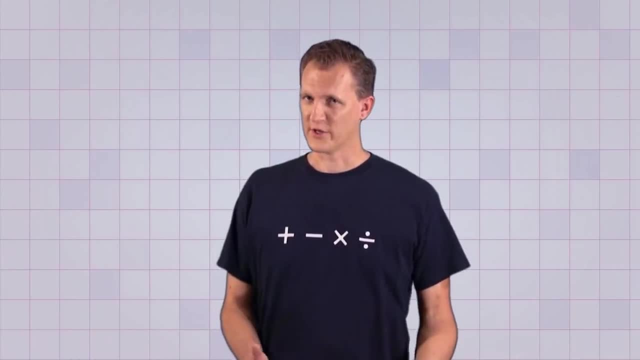 Looks like we have another one of those repeating decimals. Yep, this way's certainly easier and quicker too, But it's important to know how to do it both ways. The 5 fractions that we've just converted are so common that it's a good idea to memorize their decimal values. 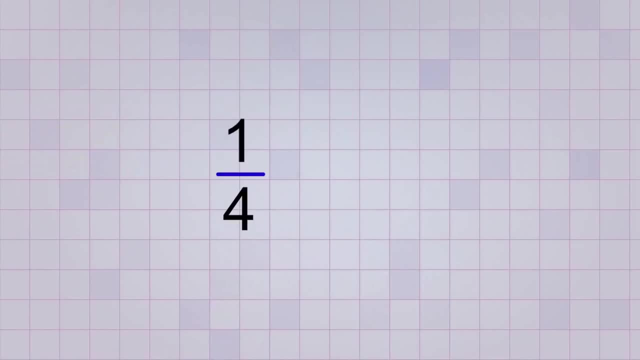 Here they are again, so you can review them: 1 fourth equals 0.25.. 1 third equals 0.33333.. 1 half equals 0.5.. 2 thirds equals 0.66.. 3 fourths equals 0.75.. 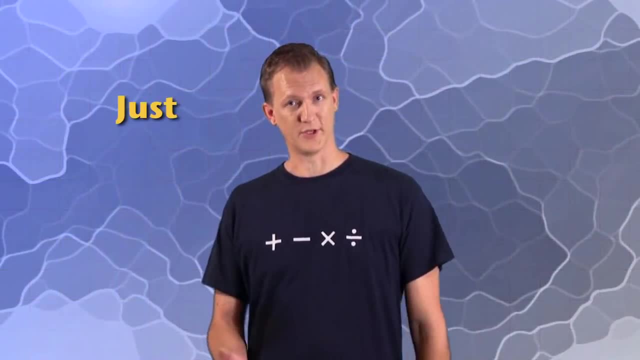 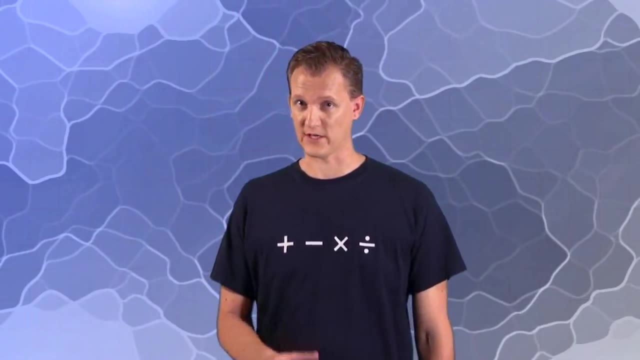 So that's how you convert any fraction into a decimal: You just divide, And we already learned how to go the other way- to convert a decimal into a fraction- in the last section, so be sure to review it if you need to. In the next section, we're going to learn a few tricks.